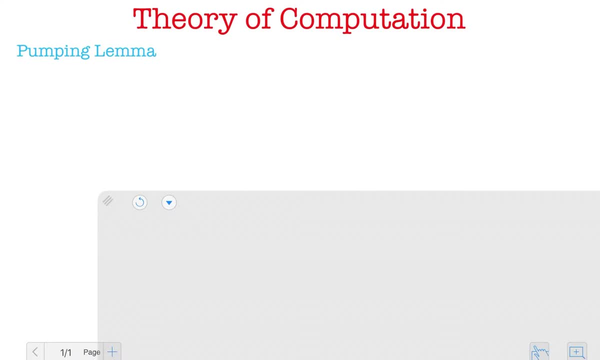 this time. the rest of it remains the same, but it says that I can split s, which is any string in the context-free language. I can split it into u, v, w, x and y, and then I can pump. so what were we? 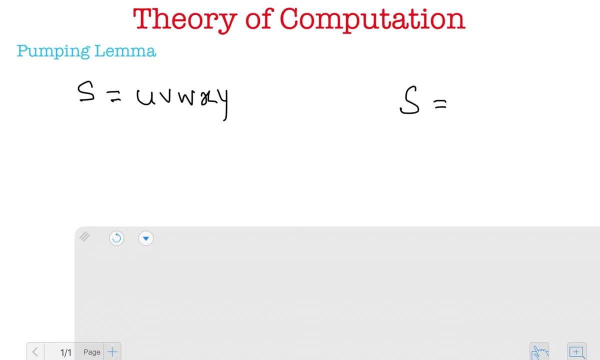 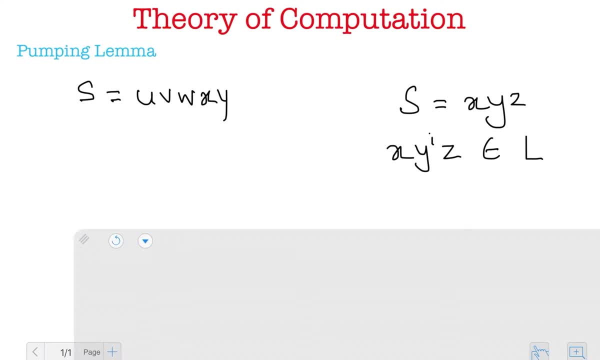 given, no matter what the value of i is, which means that we were saying that we can always find a single substring in the middle which we can pump, which we can expand. In case of the context-free language, what we say is u? v to the power. 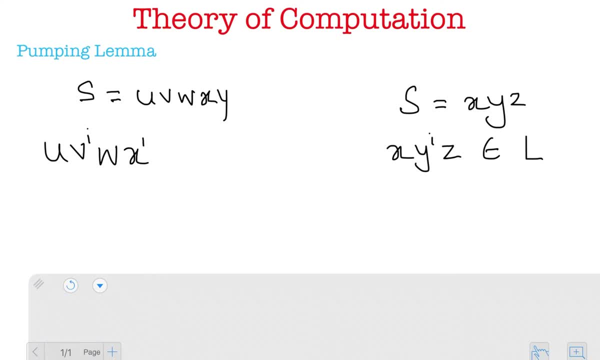 i, w, x to the power: i, y. this will belong to our language that we've been given. so all we are saying is that instead of a single substring, we can now find two substrings, and we can pump those substrings. So let's take an example and 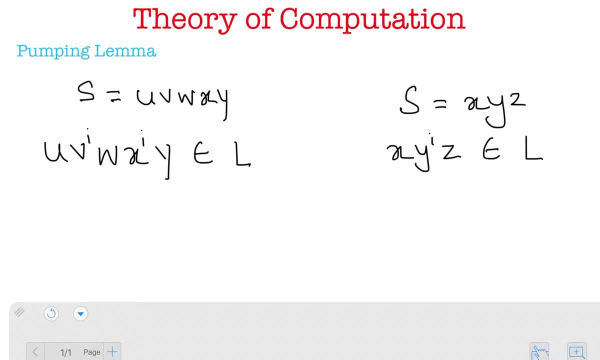 understand this. Of course, there's also a second rule change which says that my v, w and x- the length of all of these together- should be less than my pumping length, less than or equal to my pumping length. So let's take an example and then 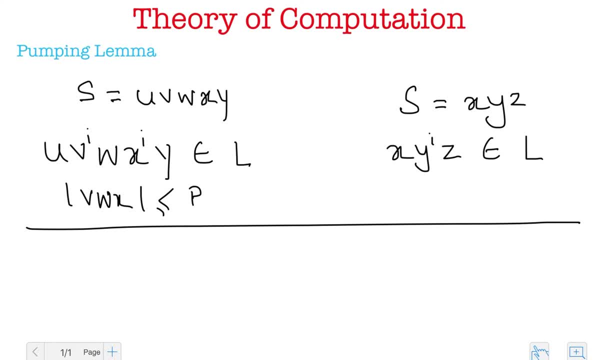 we can understand this better. So let's take our famous example of a to the power n, b to the power n. What happens now is: let's take our pumping length to be something like 3- and actually 3 might not be a great option, because I'm not going to be able to if I. 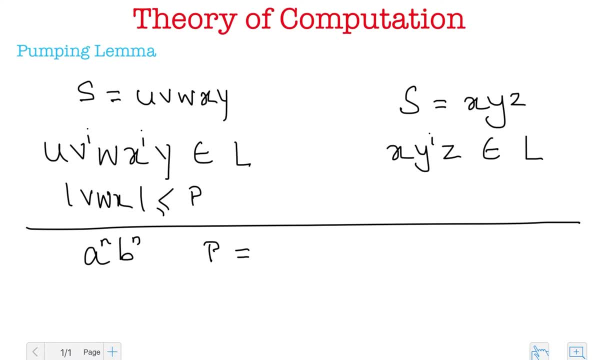 take a string of length 4, then I'll just have 4 symbols in it. I won't be able to find u, v, w, x, y, z, So let's just take the length to be 4.. Now what we can. 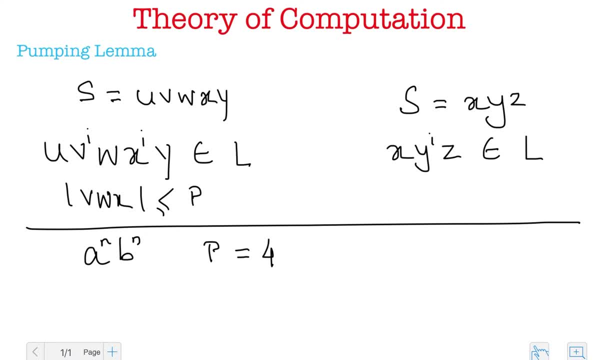 have is a string which is of length 6,. let's say So: I have a, a, a, b, b, b. Now all I have to do is I have to find two substrings and I'm going to pump those substrings. So the simple way for me to 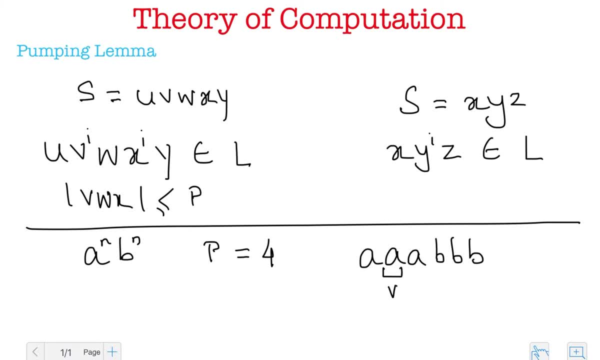 do this is to just say that this is my v and this is my x, and then I just have to put the rest of it in my u, w and y. So I say: this is my u, this is my w and this part is my y. and now when I, when I 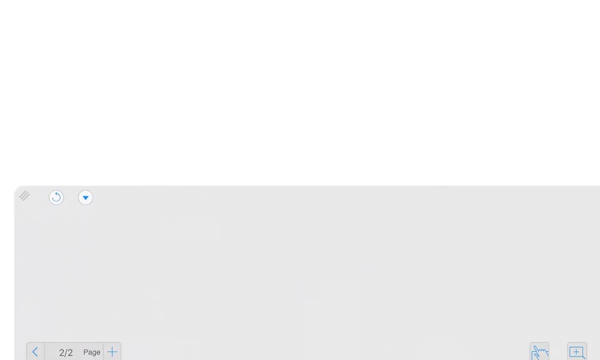 actually try to pump this. what happens is: let's just write a string again here. so I have a, a, a, b, b, b and I have: this is my v, this is u, this is w, x and y. And now when I take u, v to the power i, w, x to the power i, y, what happens is I write a, which is my u, then I have to write v, i times. what that means is: this is just going to. 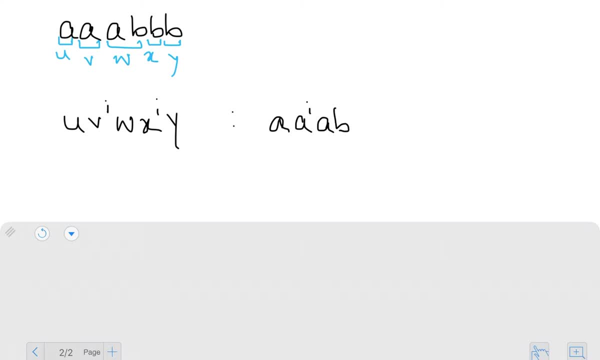 become a to the power i followed by, and an, a, b followed by b, to the power i followed by a, b. So the total number of A's and B's here has remained the same: it's I plus 2.. So that shows that this language that I've been given actually satisfies the pumping lemma. 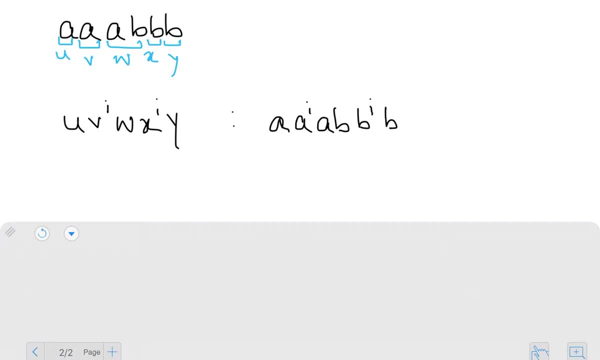 for context-free languages. Remember, though, that this is not a sufficient condition for the language to be called context-free. So, even though this follows the pumping lemma for context-free languages, I cannot say that this language is context-free, but, knowing the fact that A to the power n B to the 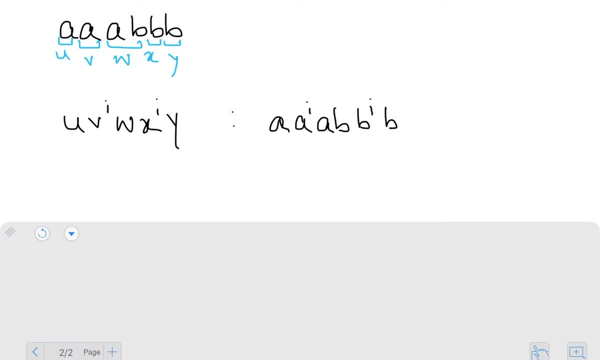 power n is context-free, I can always use the pumping lemma, which means that I know- because the language is regular, I know that it is going to follow the pumping lemma for context-free languages- What you can do, and I'm not going to get much into this.